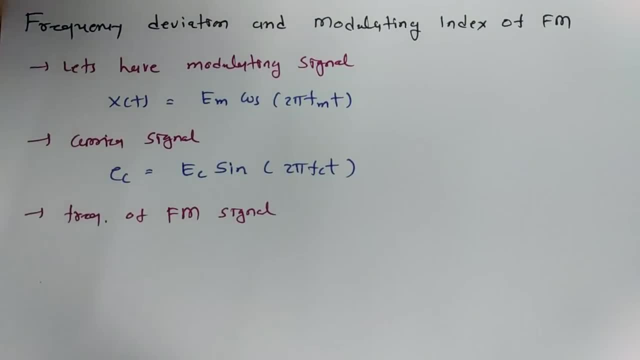 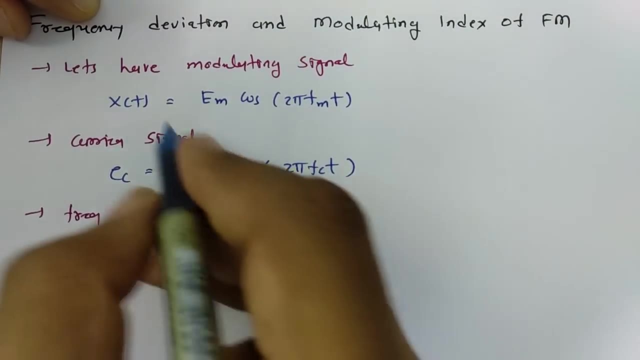 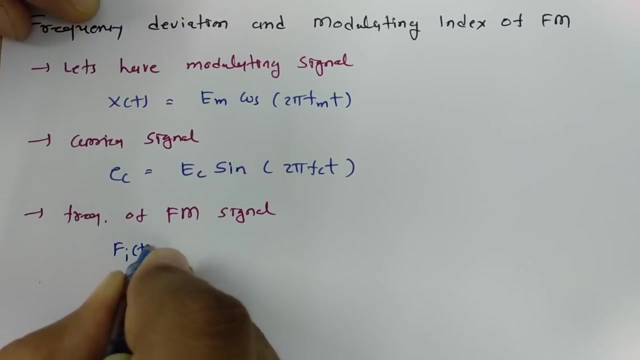 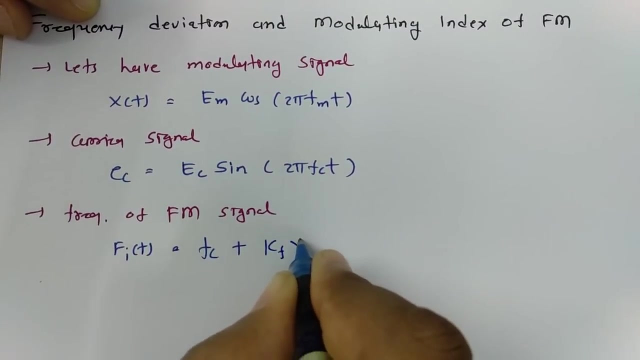 that is what varying with respect to XT. So frequency of FM signal, that changes with respect to frequency of carrier signal, FC, that changes with respect to XT. So frequency of FM signal, that is what time varying function, and if I say that is FIT, then that will be FC plus KF, XT, where KF is sensitivity of FM. 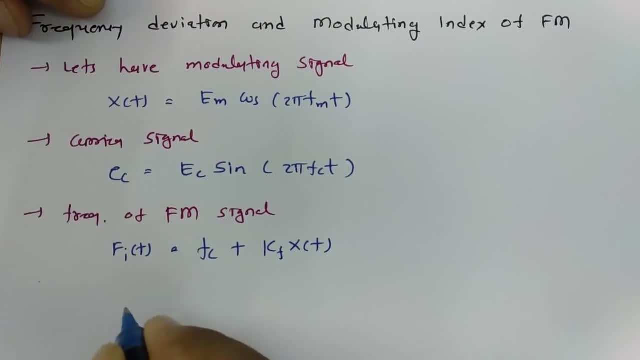 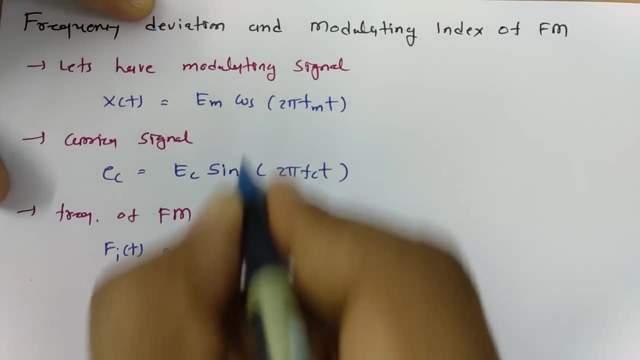 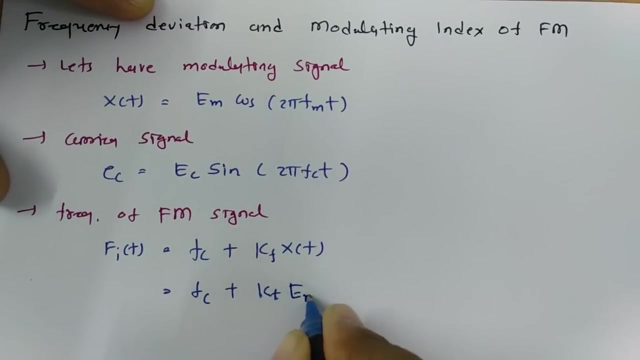 Now if I place value of XT over here, Then that will be FC plus KF. into XT is EM cos, Omega MT, where Omega M is 2 pi FM. So this will be kF E M into cos of 2 pi FM T. 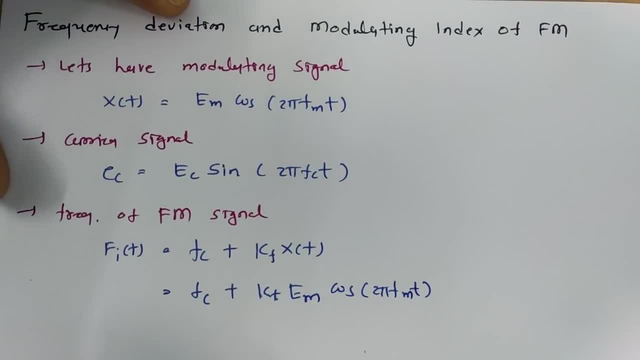 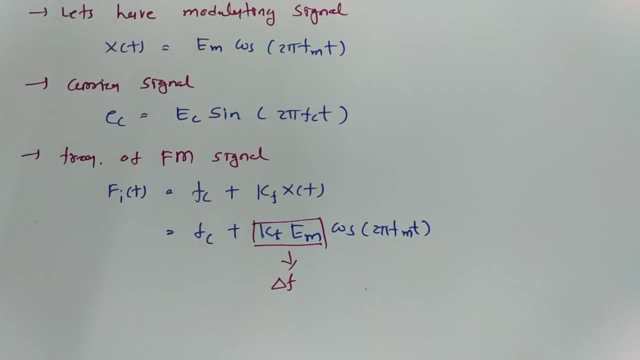 Now here, if you see the deviation of frequency, then that is what deviating with respect to this was is what maximum frequency deviation. this is what maximum frequency deviation, delta f, so frequency of fm signal that we can say fc plus delta f, cos of 2 pi fmt, where delta f 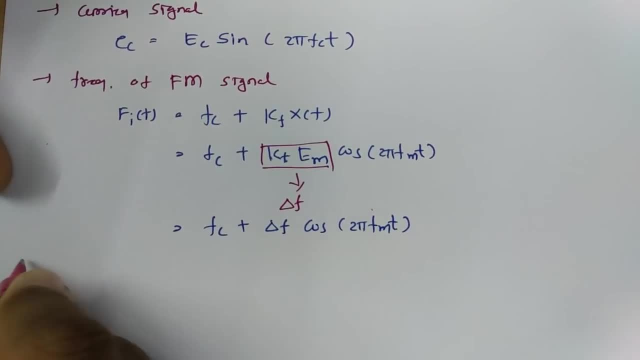 that is frequency deviation. so here, delta f, that is kf, em, that is frequency deviation. now here, what will be our maximum frequency of deviation and what will be our minimum frequency deviation? so maximum, so maximum. so maximum frequency deviation, so that will happen by fc plus delta f and minimum, that will happen. 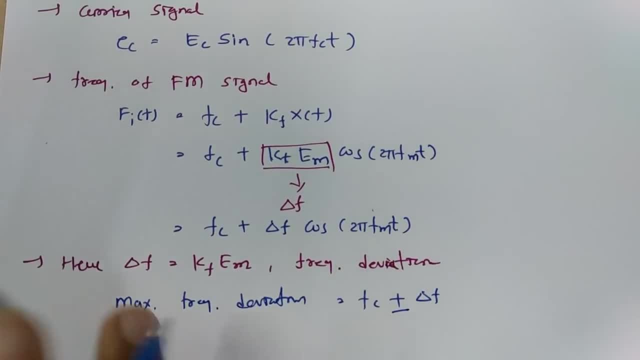 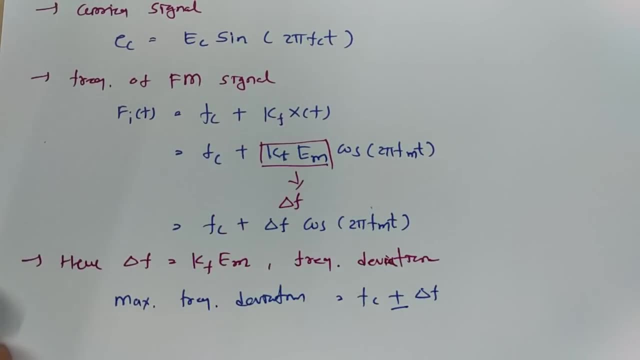 by fc minus delta f. so this is how maximum deviation will happen: where delta f is kf into em, where kf is frequency sensitivity, frequency modulation sensitivity and em, that is what amplitude of modulation. so this is what about frequency deviation. now let us derive a formula for modulating. 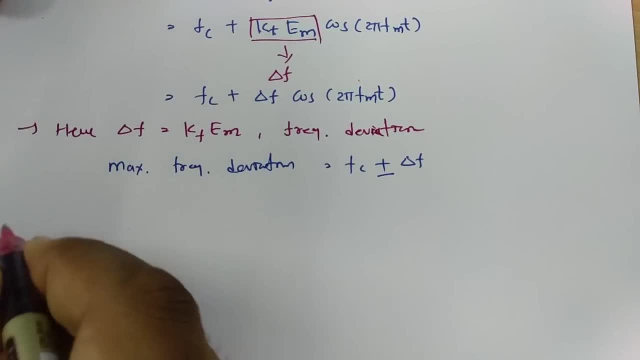 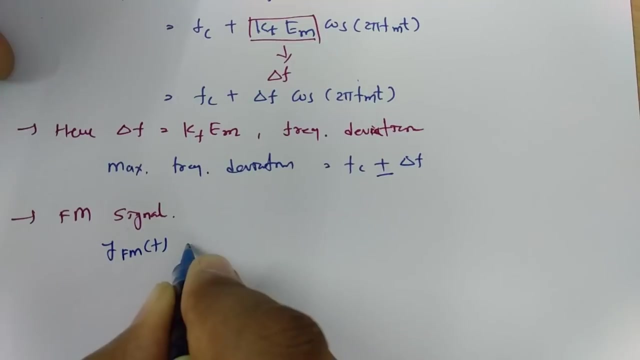 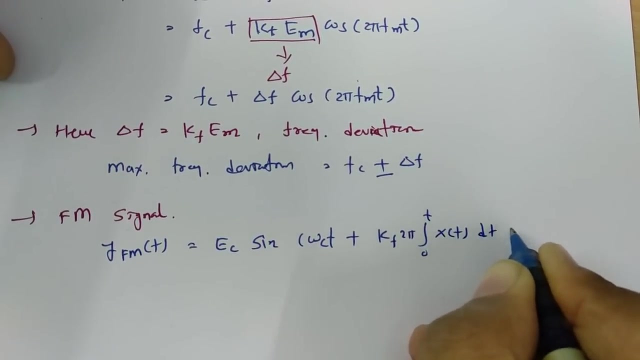 index now fm signal: fm signal that we have already seen in my previous session, so that you can see it from there where fm signal is, y of fmt that we have seen and that was ec, e, sin, omega, ct, plus kf 2, pi, integration 0 to t, xt, dt. so this is standard frequency modulated signal. 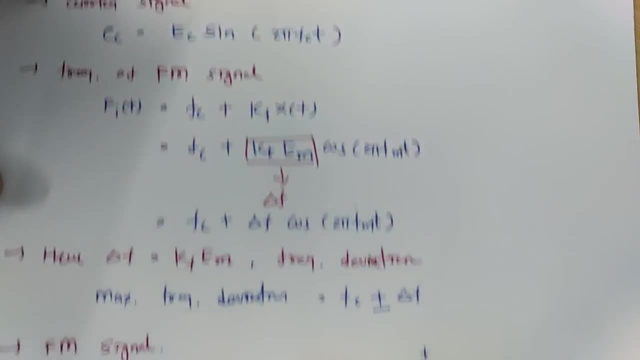 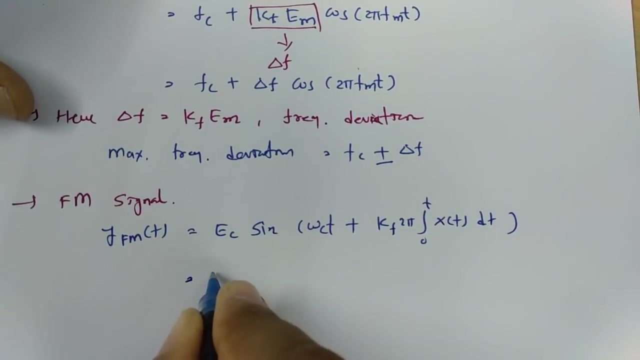 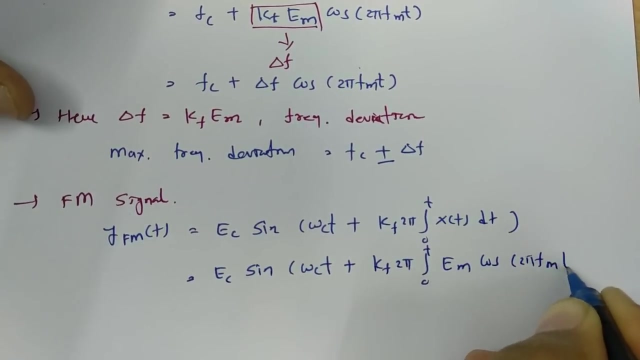 now where, if i place value of xt that is em cos 2, pi, fmt, then we can simplify that formula further. so ec, sin, omega, ct plus kf, 2 pi integration 0 to t, xt, dt. so this is standard frequency modulated signal plus kf 2 pi integration 0 to t, where xt is em cos 2, pi, fmt, dt. now if you, if you do this integration, 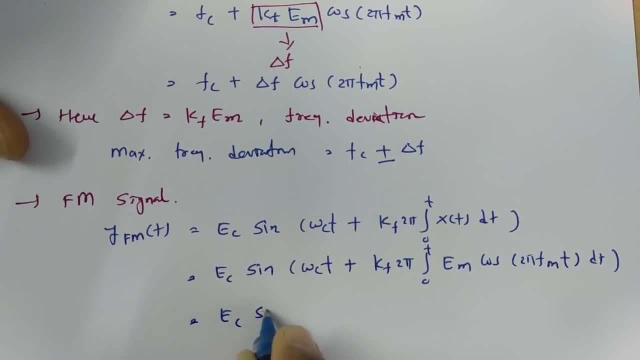 then we'll be simplifying this equation further. so em, that is constant. take it outside. so kf, 2 pi into em, and integration of cos, that is sin, and this is the constant that we have here. so we have, this is what constant that we need to divide. so, divided by 2 pi fm into sin of 2 pi fmt. now, 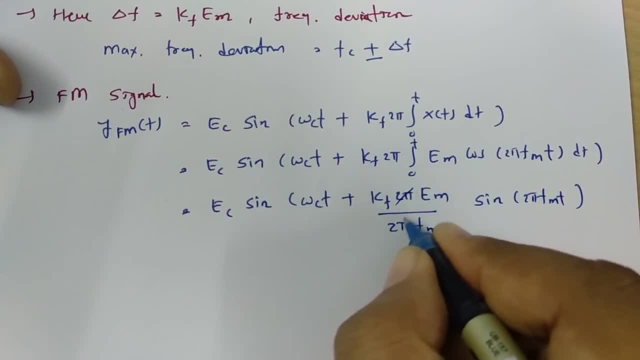 here 2 pi. that will get cancelled. so we will be getting this equation as ec sin omega ct plus kf em divided by fm sin 2 pi fmt. so we will be getting this equation as ec sin omega ct plus kf em divided by fm sin 2 pi fmt. you should have to devise it as an international量 correlation, but now we can operate with this equation. this equation will do JEFC不到. 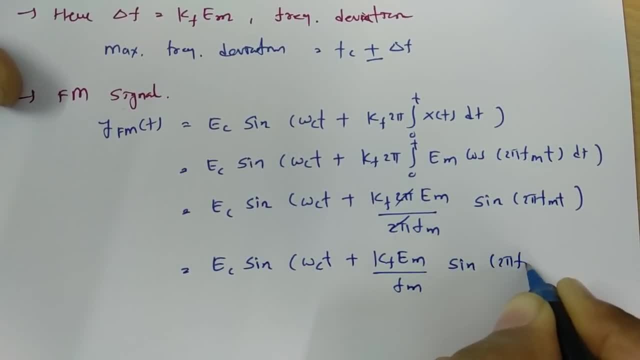 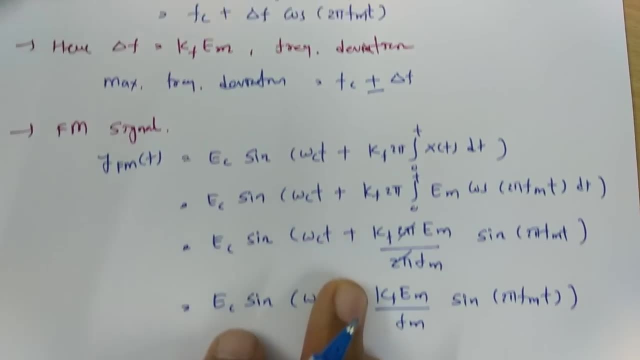 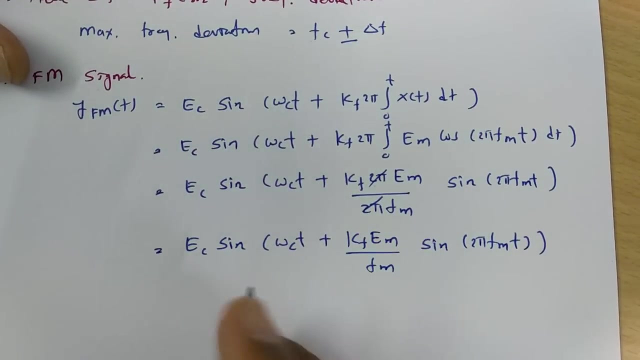 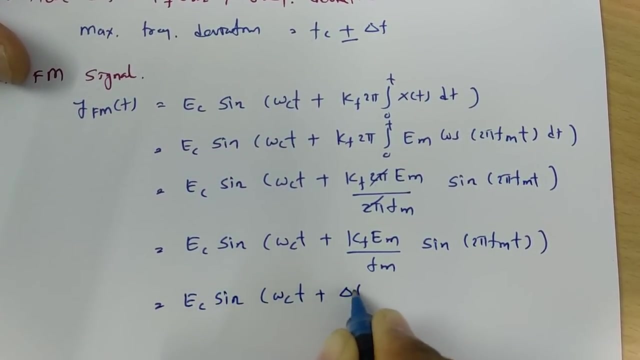 fm sine 2 pi fmt. now here, kf, em. that is what frequency deviation you can see. kf into em, that is frequency deviation, so just place that over here. so it will be having ec sine omega, ct plus delta f divided by delta. delta f divided by fm into sine 2 pi, fmt. now here: delta f by fm delta. 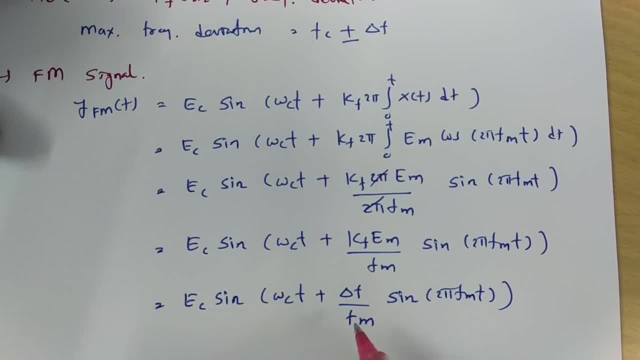 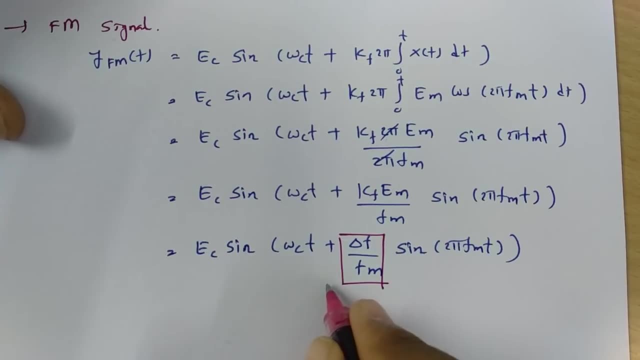 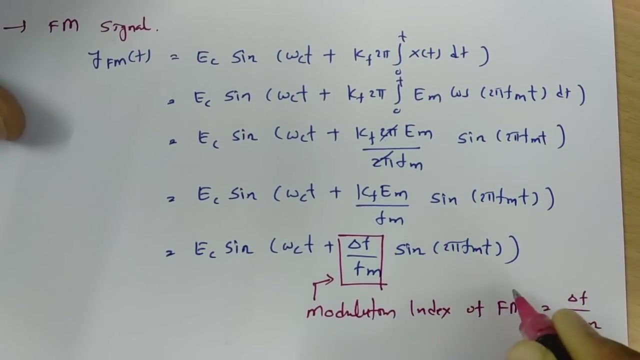 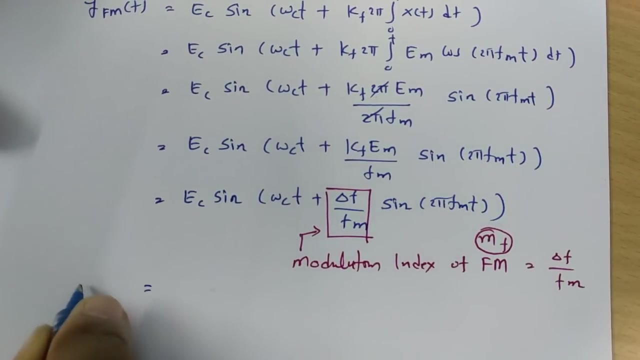 f is what frequency deviation, and fm, that is maximum frequency of modulating signal. so this is modulating index, this is modulation index of fm, that is delta f by fm and we note it by mf. so mf, that is what modulating index, that is delta f by fm. so fm signal that we can even represent by pi of fmt, that is ec sine omega ct. 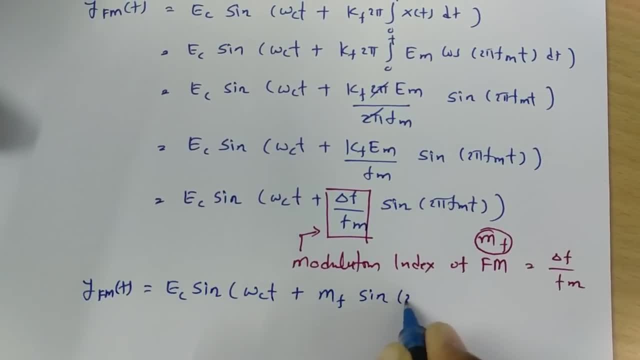 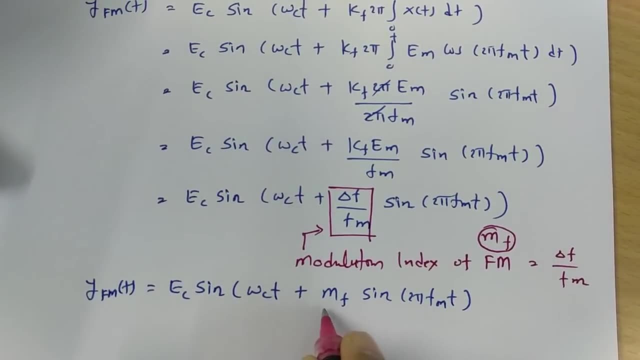 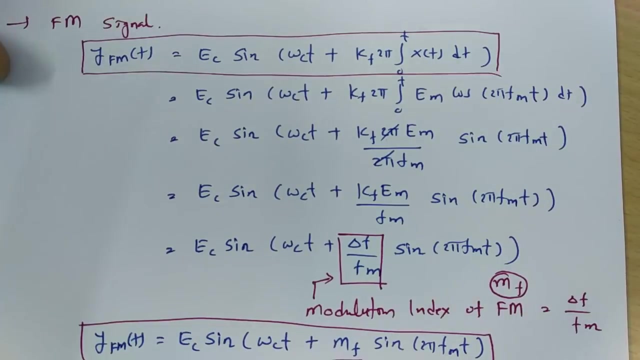 plus mf, sine, 2, pi, fmt. so this is what about modulation index and this is how we we can represent fm signal. so this is fm signal and second way of representation of fm signal is like this: so these two basic equations, these are frequency modulation in signal. 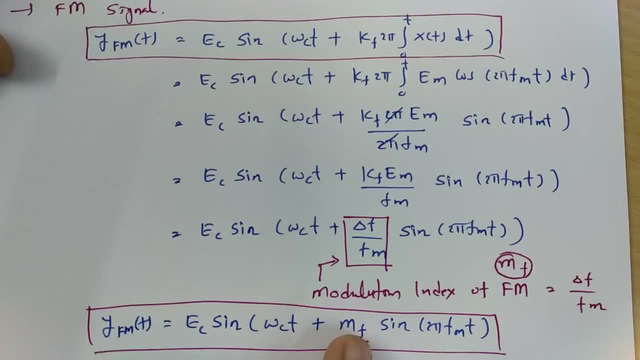 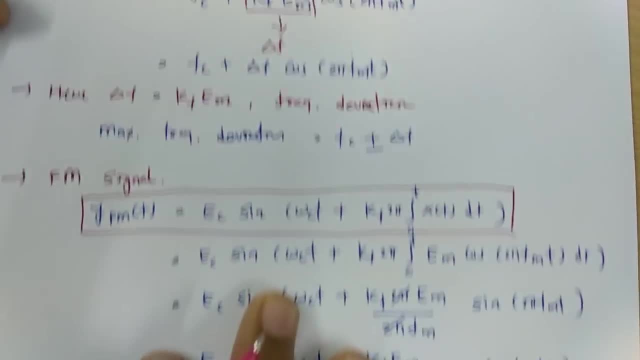 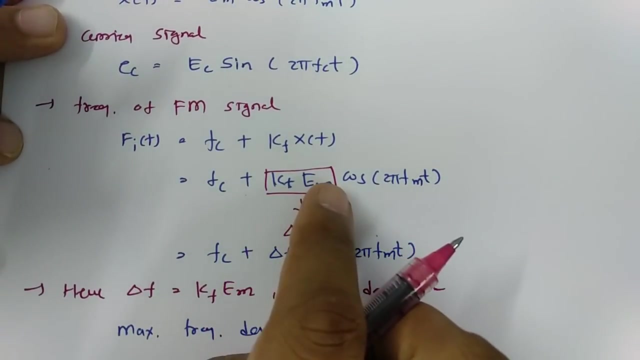 and where you will be finding this mf, that is modulation index, that is delta f by fm. So two things that I have told you, like I will be explaining that in this session. One is frequency deviation. So frequency deviation, that is frequency sensitivity into em, and second is 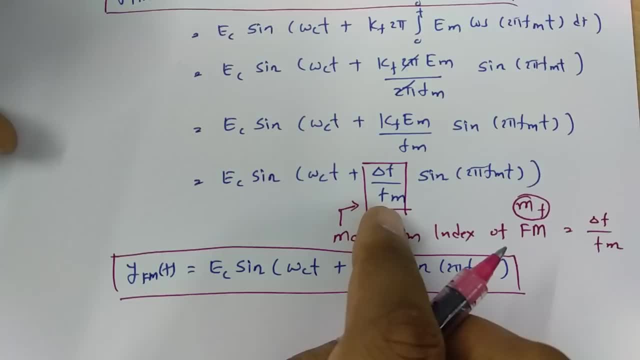 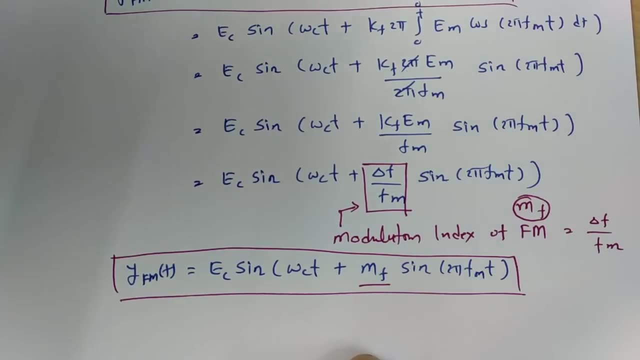 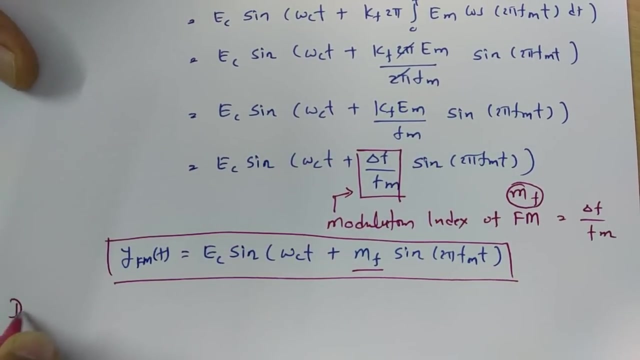 modulation index, that is delta f by fm, where delta f is frequency deviation. Now there are two more basic definitions that even we need to understand. One is deviation ratio. So deviation ratio, that is maximum deviation divided by maximum modulating frequency. So deviation ratio is maximum deviation divided by maximum modulating. 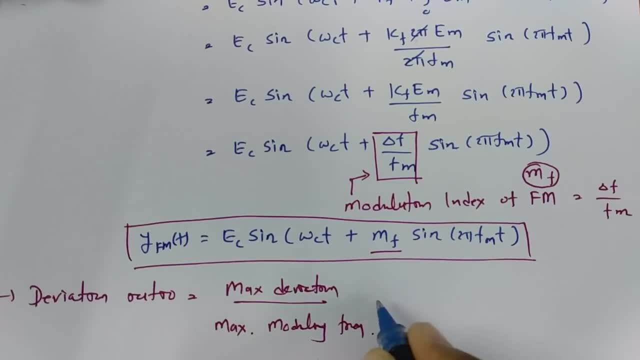 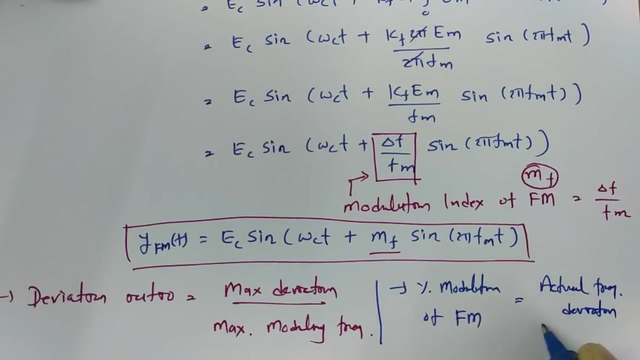 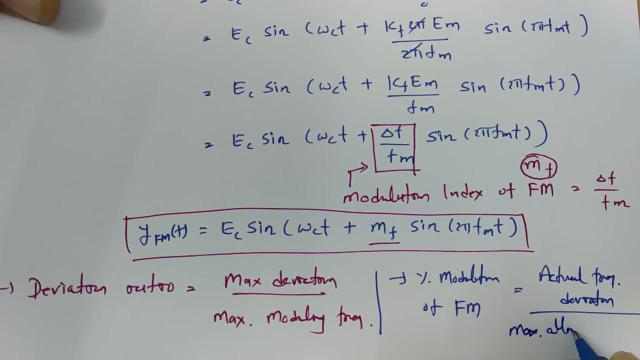 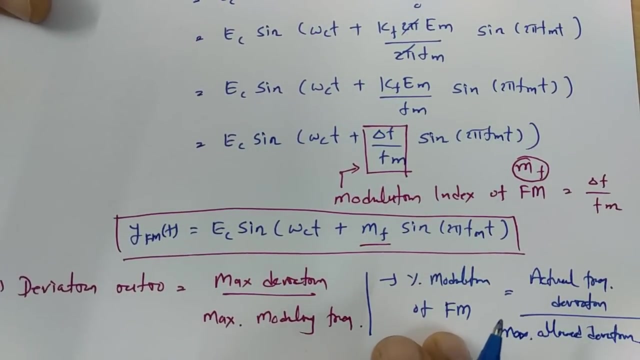 frequency and second basic definition that one should know, that is percentage modulation of fm. and percentage modulation is actual frequency deviation divided by maximum allowed deviation. So from that we can calculate percentage modulation of frequency modulation, Percentage modulation of frequency modulation, that is actual frequency deviation divided by maximum allowed deviation. 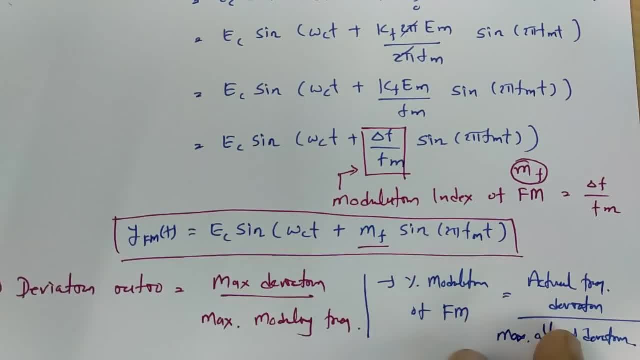 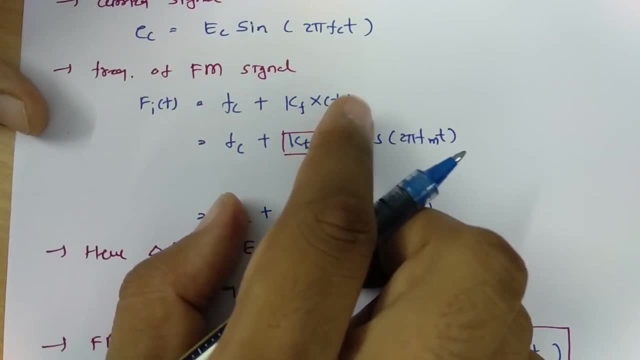 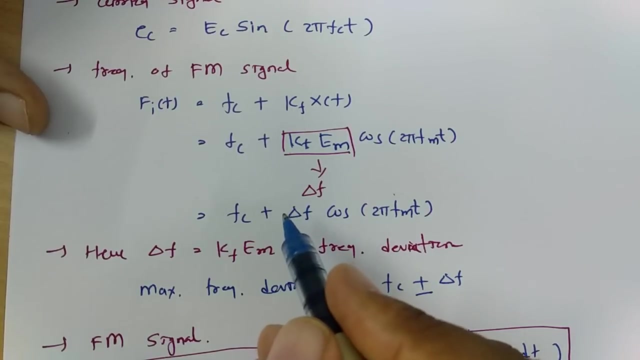 Now here one can see this actual deviation that is happening. as per this function, fit is equals to fc plus kf, xt, where xt is time varying function. So obviously maximum deviation will be kf into em. So that is delta f and actual deviation that will vary with respect to time, like this cos of 2 pi fmt. 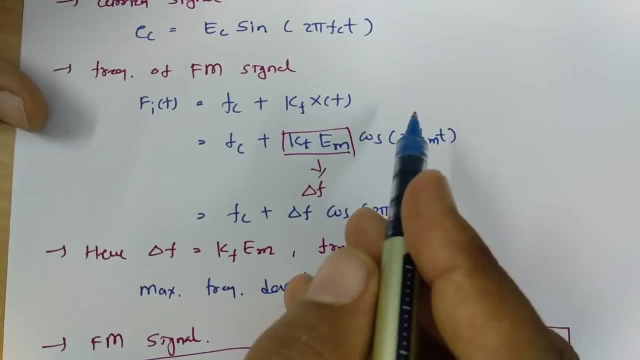 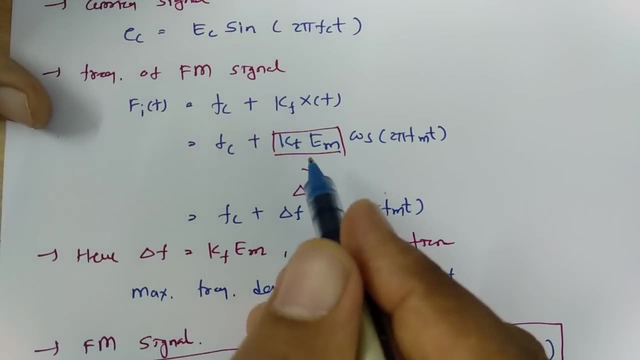 So, based on modulating signal, we will be having actual deviation and maximum deviation is frequency sensitivity. So that is how we'll be having frequency deviation delta f, and that even varies with respect to time. So this is how it varies with respect to time. 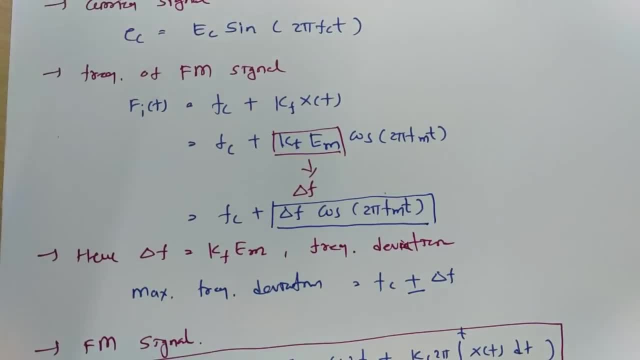 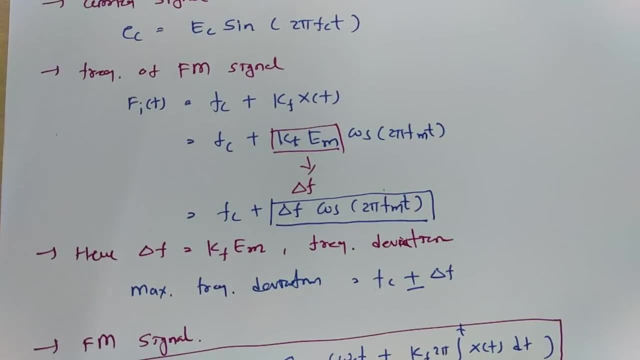 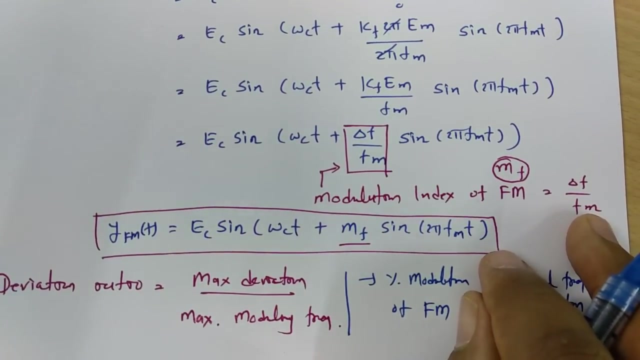 So here, few basics that we need to understand. What is frequency deviation? Frequency deviation is kf into em and what is modulation index? so of fm, so that is delta f by fm, And when we talk about deviation, that is df by fm. So we are talking about the deviation from xt into fm. So trick is that kf into em divided by maximum xt into fm is equal to kf feelings for duration of the interval. So that is how we will talk about this. 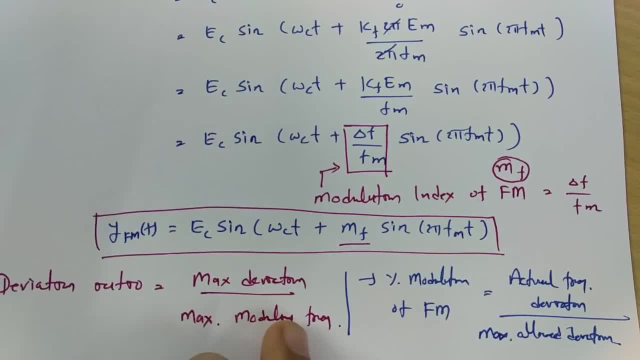 ratio. so that is maximum deviation divided by maximum modulating frequency and percentage modulation of fm. that is actual frequency deviation divided by maximum allowed deviation. So this is how we can calculate frequency deviation and modulating index of fm. Thank you so much for watching this video. You can give me your valuable suggestions, Your suggestions. 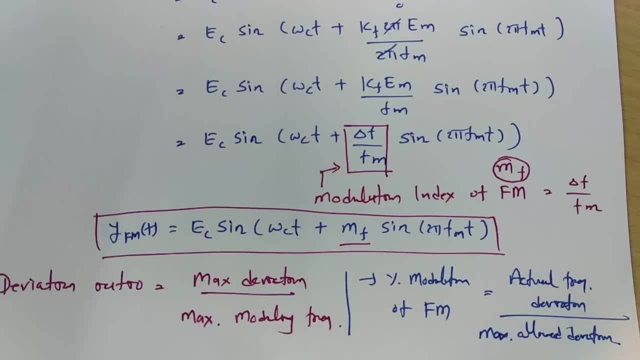 are most welcome to me and based on your suggestions, definitely in future I will be releasing videos and in next few sessions you will be finding few more basics of fm and then after I will solve examples based on fm and I will be solving all examples related gate examination. So I will be covering gate examination course as well as course of university.